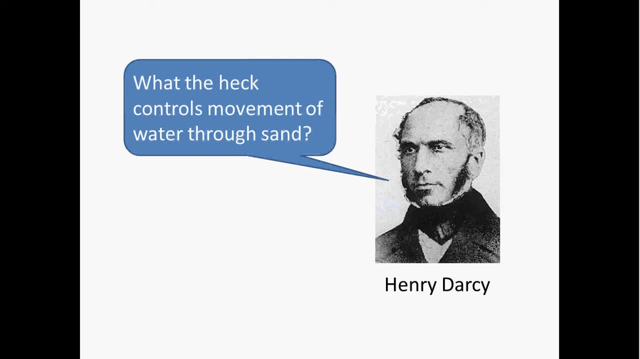 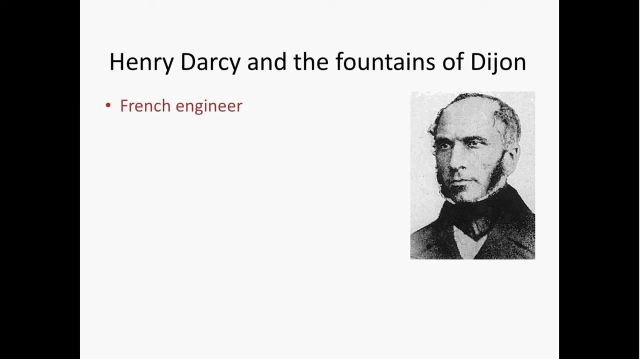 what the heck controls the movement of water through sand, And I imagine that we've all asked that question a time or two, Although he probably would have said it in French because he was actually a French engineer. Just to give you a little bit of historical context on this topic. 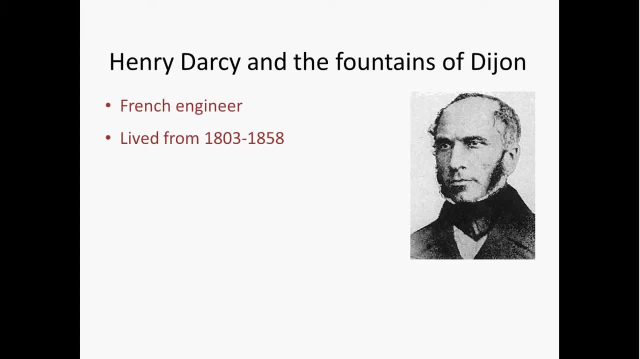 he was an engineer and he lived about the same period of time as Abraham Lincoln. During his life, he was very famous for bringing a water distribution system to Dijon in 1840. This was a big deal, because very few places at the time had water distribution systems. 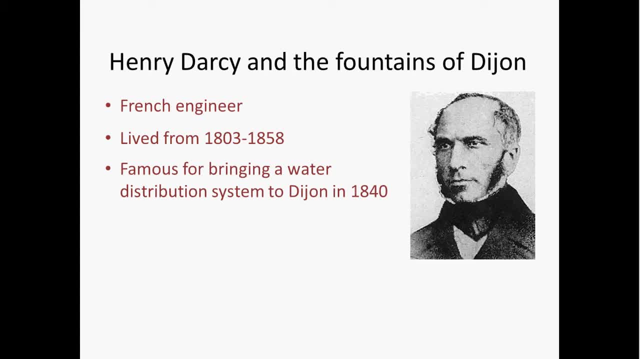 It wasn't. It was also at this time that few places had sewer systems, So if you were living in a city, a good, reliable source of clean water was really important. For reference, Paris didn't have a water system distribution system until 1865, a full 25 years after the little city of Dijon got. 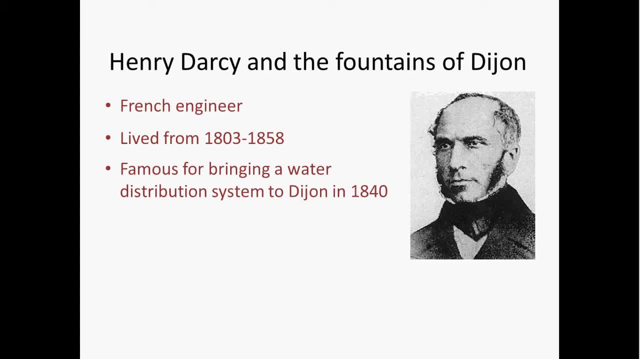 its water distribution system. it wasn't until very late in his life, about two years before he died, that he carried out the experiments that perhaps he is best known for today. he performed the experiments in a hospital, and I might seem like a really odd choice, but at the time there probably weren't many places. 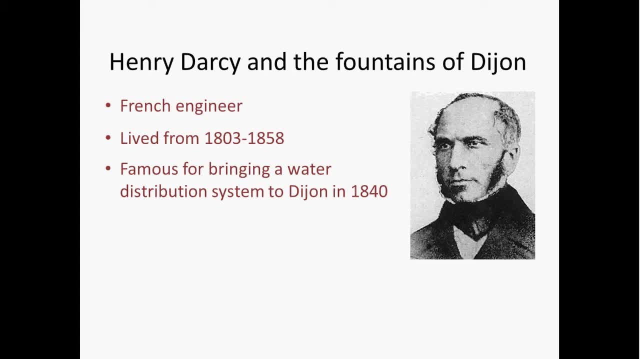 where that were, you know, convenient for setting up experiments. the experiment that he performed, he published the results in this report in 1856 and they were just described in a couple of pages in the very back of the report, I think, one of the appendices for the for the report. so it was very much just an 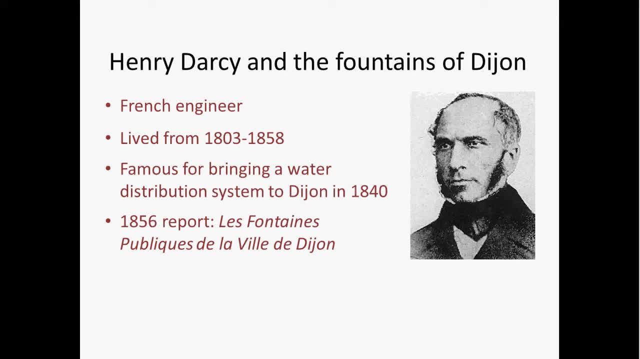 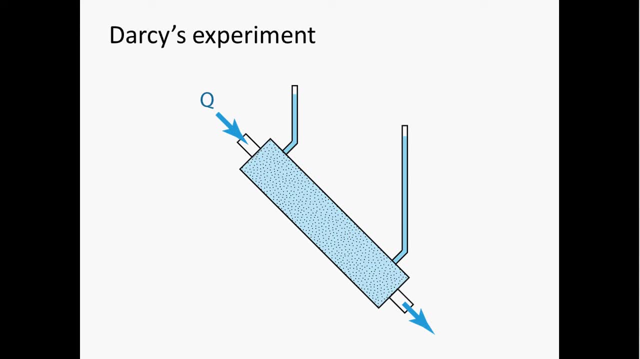 afterthought, but it turned out to be a really useful and important piece of work. so what we're going to do today is we're going to talk about the biochemistry of the reason why it was first announced. so what we're going to do now is walk through some aspects of Darcy's experiment. this will help. 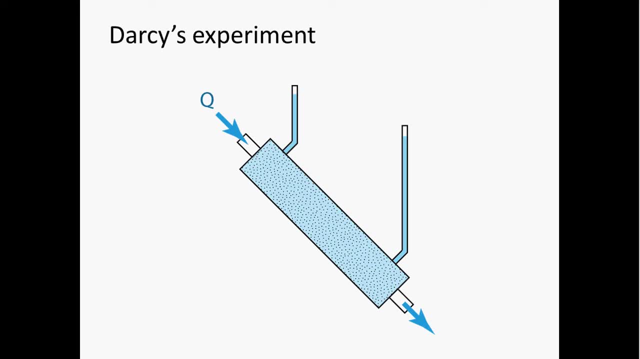 illustrate some basic controls on the movement of water through porous medium and also the process of science, how you can apply some basic reasoning, collect data and then figure out relationships. so what Darcy did was set up a tube that contained some sand, and that tube had some smaller tubes in it, called 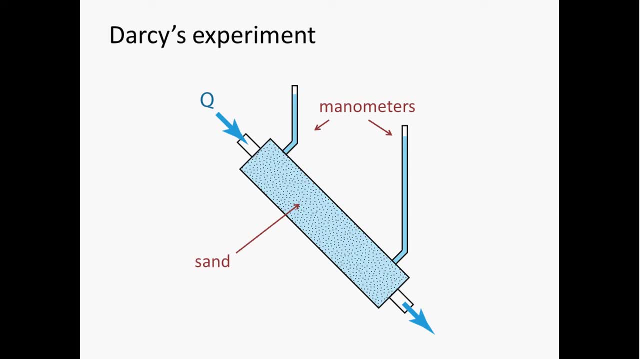 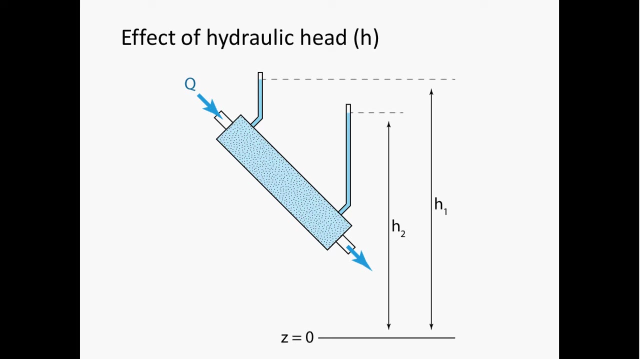 nanometers, poking into the near the inflow and outflow in, and he flowed water through the sand tube and observed how different variables affected flow. Hydraulic head is the name given to the height that water rises in the manometers relative to some arbitrary datum. 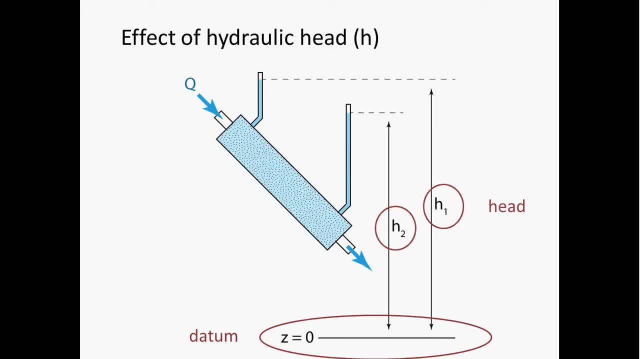 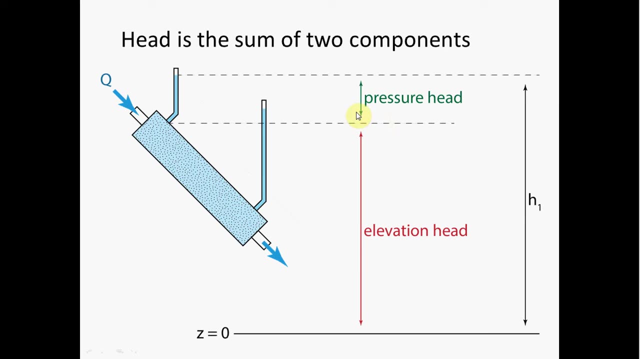 In natural environments we would typically pick sea level to be the datum In a lab experiment. you might just pick the bench top where you're carrying out the experiment, because it's more convenient. Hydraulic head is the sum of two components the height that water rises in the tube. 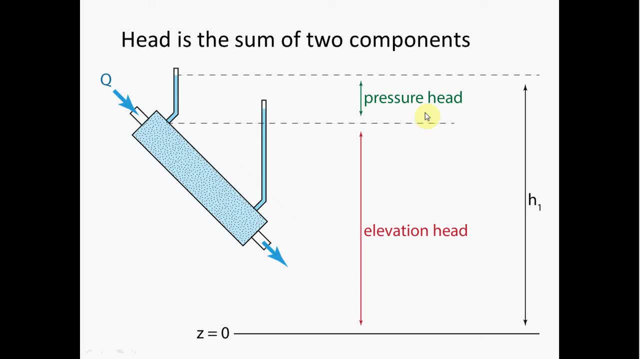 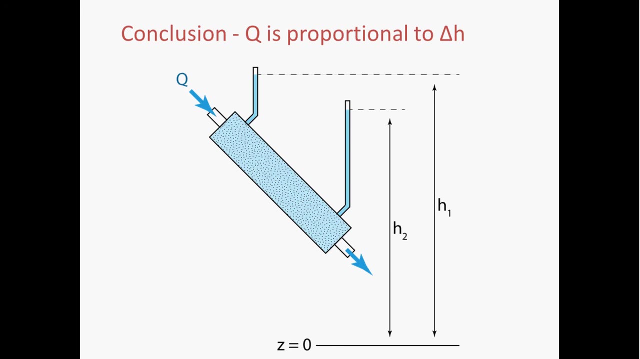 as a result of water pressure. we call that pressure head and then the height that the water has because of how far the tube is above the datum. Okay, so that would be elevation head. What Darcy observed was that water always rises in the water. 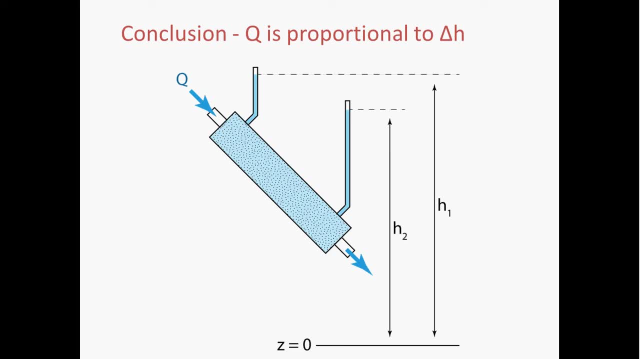 and that water always flows from high head to low head and that the rate of flow through that sand tube is proportional to the difference in hydraulic head measured between the manometers, In other words delta H. The difference between this hydraulic head and this hydraulic head is delta H, right here. 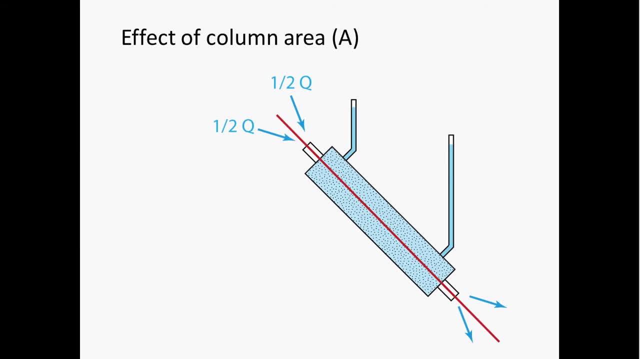 Okay, how about column area? How would this affect flow? Well, this is really straightforward. Basically, if you were to put a partition in the column such that the area available to flow was divided in two, the flow rate through each half of the sand tube. 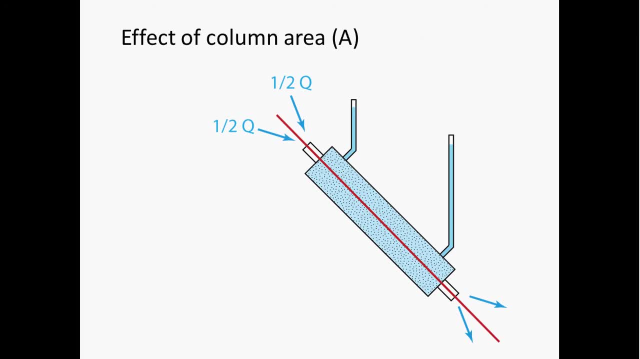 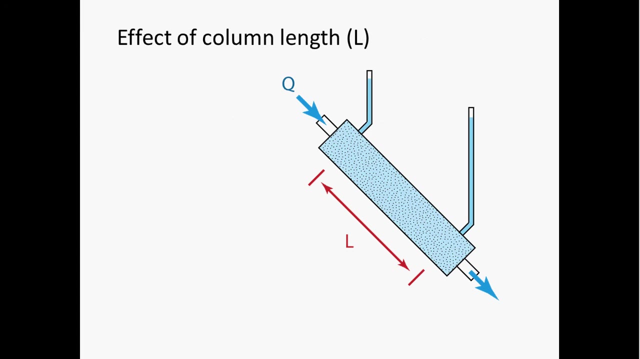 would be equal to one half of the total flow. Okay, so from this, Darcy concluded that the rate of flow is proportional to the area of sand available. Lastly, what about the length of the tube? Well, Darcy figured out that if you keep 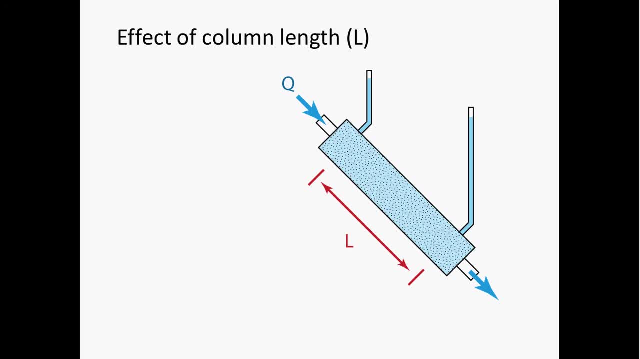 the head difference between each end of the tube the same, but you lengthen the tube, it affects the flow rate. okay, So imagine, in fact it causes flow rate to decrease. Imagine that this sand tube is one foot long and that the difference in head is six inches. 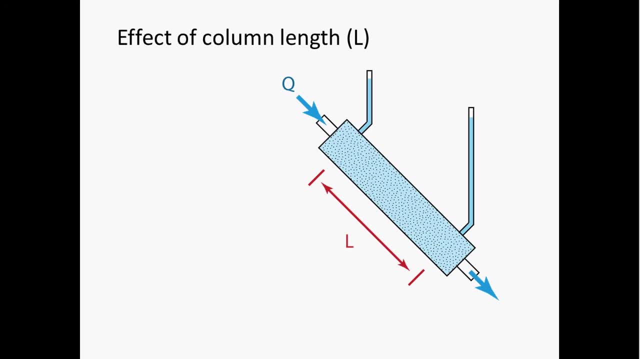 Okay, that's a pretty steep change in hydraulic head over the length of that tube, All right, and so water would want to flow through that fairly quickly. But if the tube were 10 feet long, that six inch drop over 10 feet isn't nearly as steep. 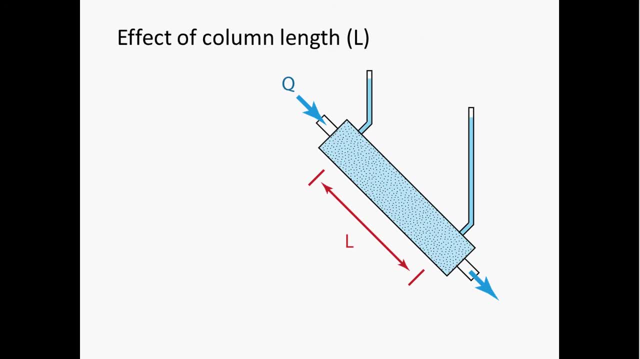 In that case, the water wouldn't move through as fast. Okay, so from this we can conclude that the length that flow through the tube is inversely proportional to length. In other words, if all else is the same, as length increases. 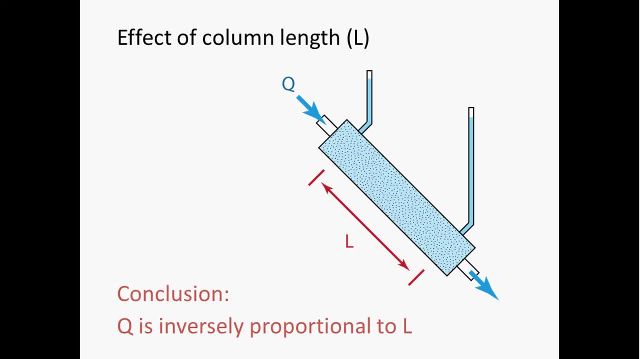 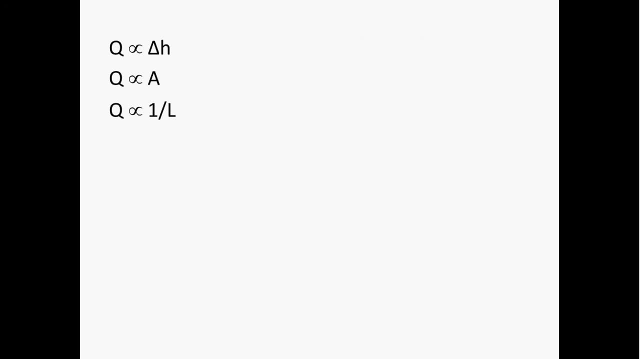 flow decreases. Okay, so these three lines summarize what we've just discussed. Flow is directly proportional to the difference in hydraulic head between each end of the tube, It's proportional to the area of the column and it's inversely proportional to the length of the column. 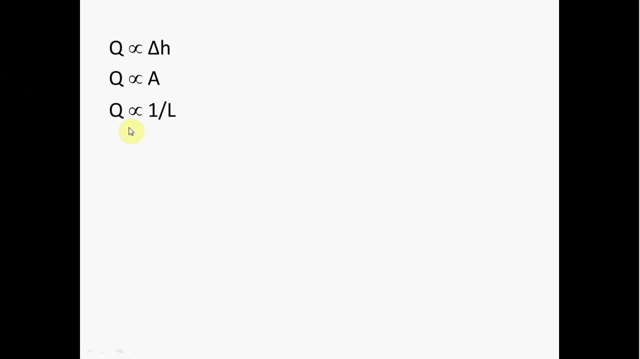 Okay, this symbol right here means proportional, So this means inversely proportional, because one over L. So if we put this together, this is what we get. Now we can replace this proportional sign with an equal sign by adding a constant of proportionality, K. 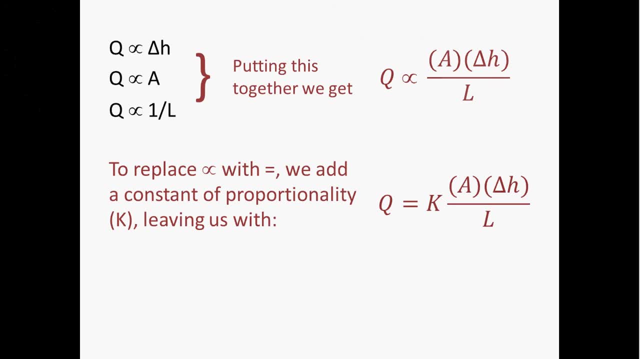 And when we do that, this is what we get. Okay, and if we just rearrange this a little bit, we end up with this form of the equation, And that is Darcy's Law. So it really is not that complicated. 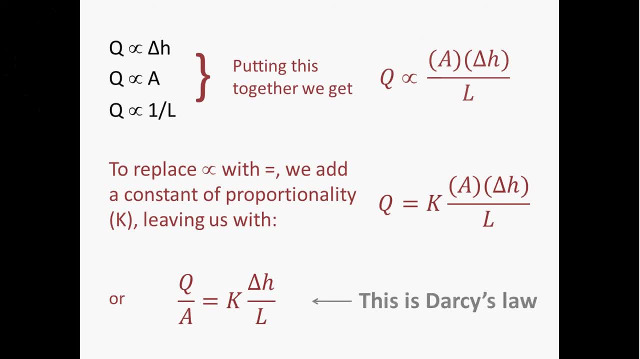 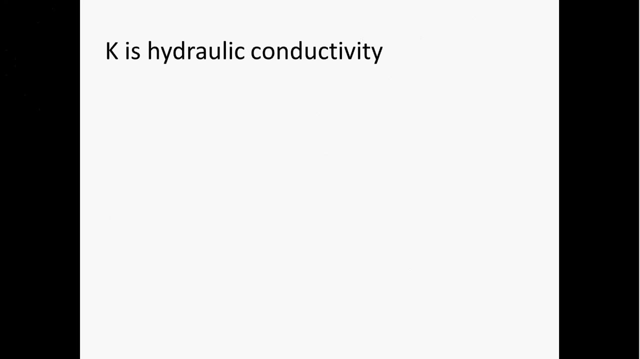 If you understood each part, each of the parts that we went through in the previous slides. this just combines them all into one equation. One of the things that might seem a little mysterious is this: K. What the heck is K? Well, K is hydraulic conductivity. 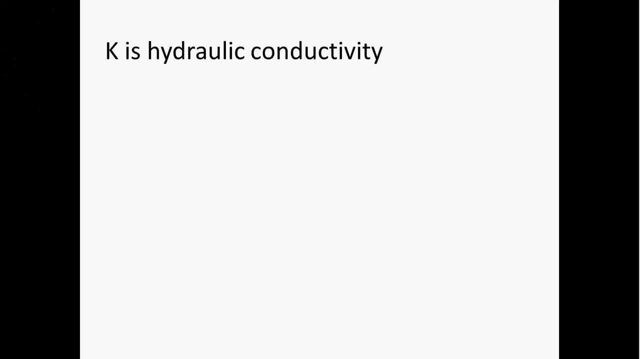 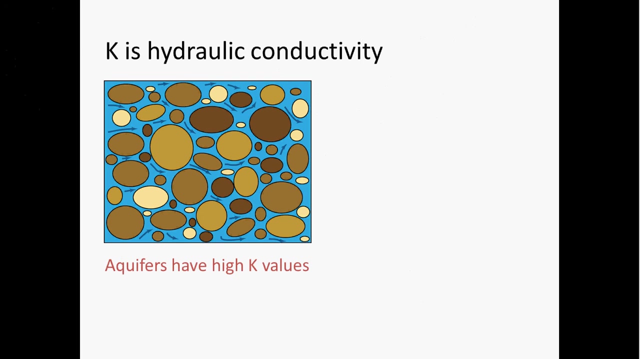 So let me explain this a little bit Basically. you can think of it as you know, basically the same thing as permeability. It's a little bit different, but think about it as permeability. Aquifers have high hydraulic conductivity because they can transmit water relatively easily. 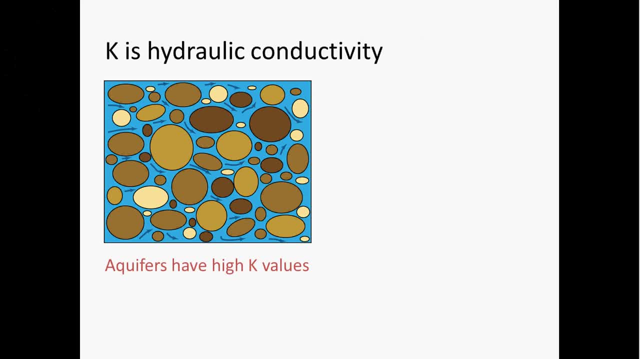 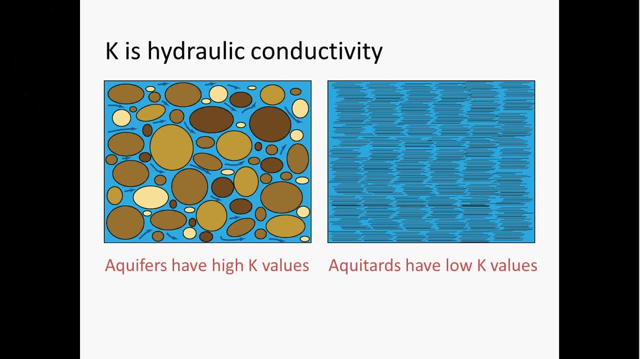 Water can flow through them. They're fairly permeable. Aquatards have low hydraulic conductivity. They're relatively impermeable. Water does not flow through them very easily. In reality, hydraulic conductivity is a little bit more than permeability. It combines permeability with properties of the fluid. 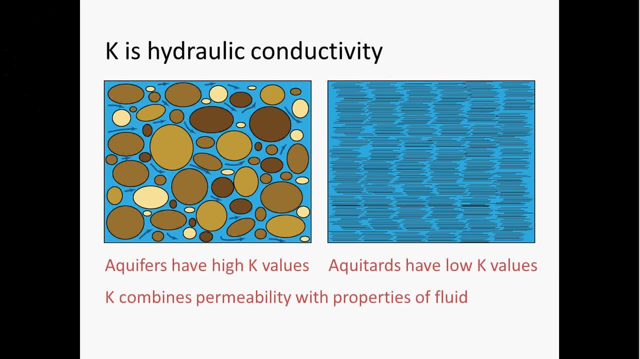 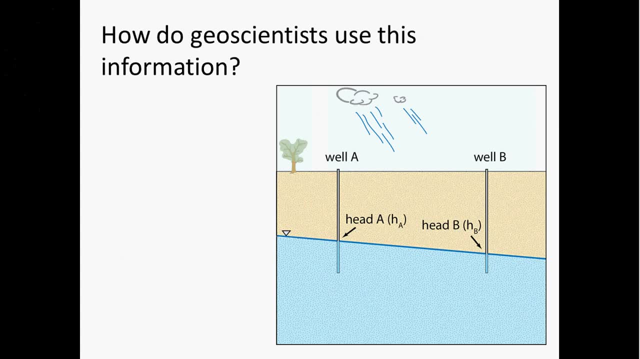 But in any case, just think about it as a measure of how easily water can flow through a porous medium. Okay, so how do geoscientists use Darcy's Law and this information that I've just given you? Essentially, you can think of wells. 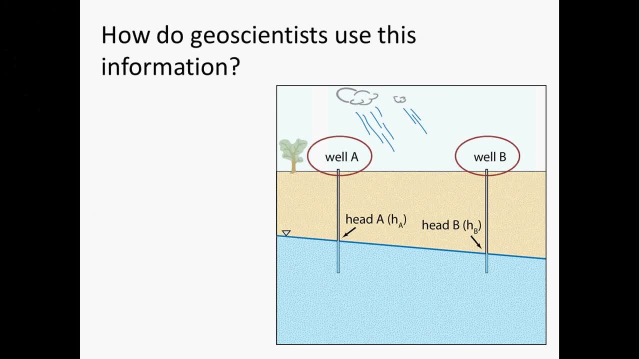 as the same thing as those manometers. They fill the same role as the manometers I showed you in Darcy's experiment. So we can go out and measure the elevation of water in a well and that tells us the hydraulic head where that well is open in an aquifer. 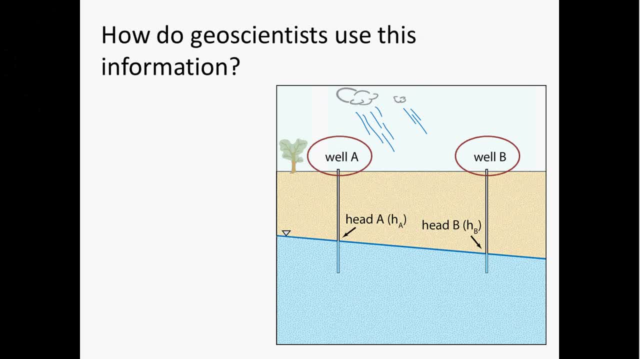 So we can use these measurements to help determine what direction groundwater is flowing in an aquifer. Okay, so in the illustration shown here, this simple illustration, we would conclude that groundwater is flowing from the left to the right towards well B, because hydraulic head decreases. 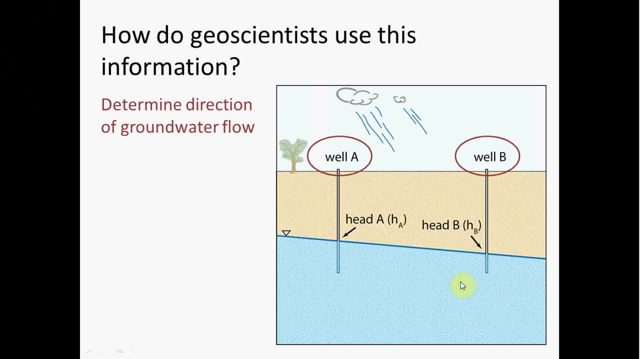 in that direction. The groundwater always flows from high head to low head, Okay, And we can use this to help understand flow rates. by assessing groundwater flow and combining it with knowledge of geological properties of aquifers, We can evaluate how much water is available in aquifers. 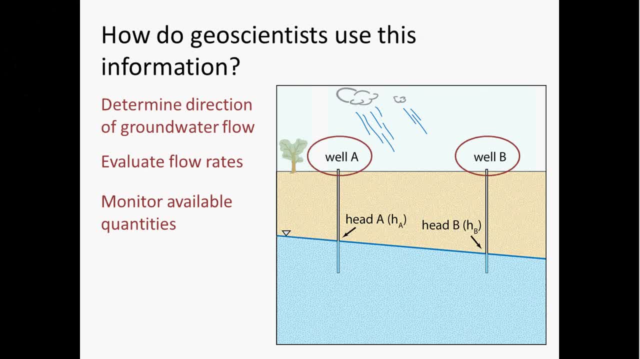 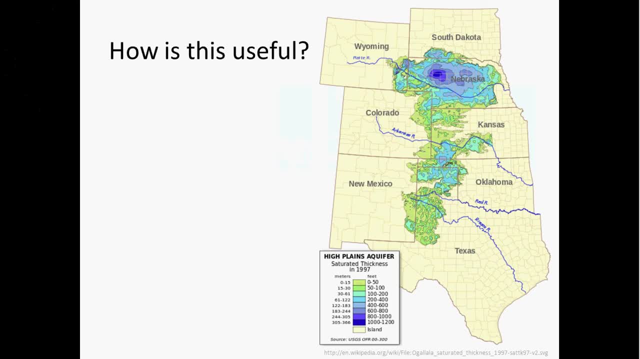 and how that changes over time. Okay, How do we use this? How is this useful? Well, given the extent to which we rely on groundwater as a source of drinking water and irrigation water, this information is extremely important because it helps us manage critical water resources more. 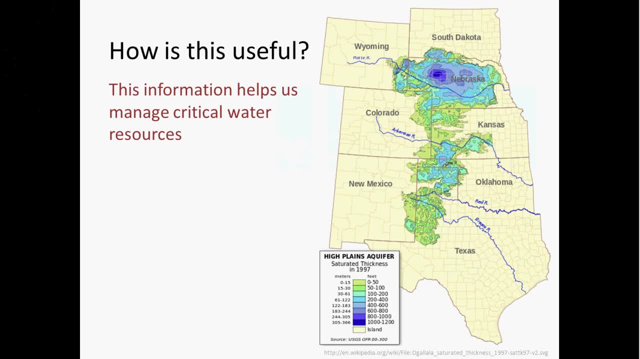 effectively, and this is a huge, this is a big deal. It's really important. These water resources are extremely important, so we need to be able to manage them effectively. One of the examples that I'm going to focus on in the next lecture is shown here.